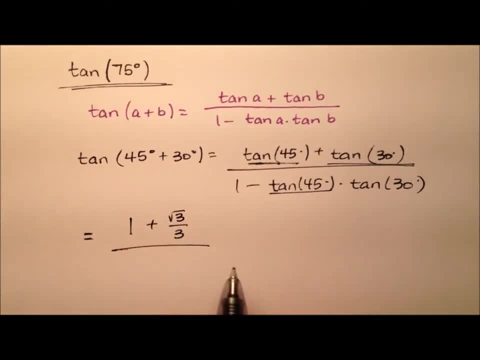 plus radical three over three, and then for my denominator it'll be one minus and then one times. So really it's just going to be this guy right there. Okay, it looks like we have a nice complex fraction, So it's a fraction overall. 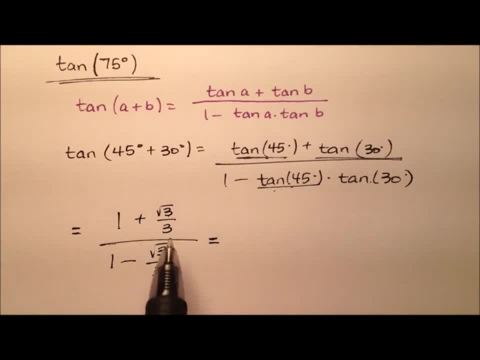 but the numerator and denominator both contain their own fractions, So let's go ahead and get common denominators on top and bottom. So it looks like I'll have three plus the square root of three over three and three minus the square root of three over three. 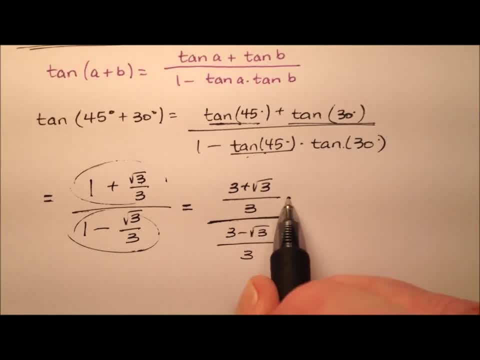 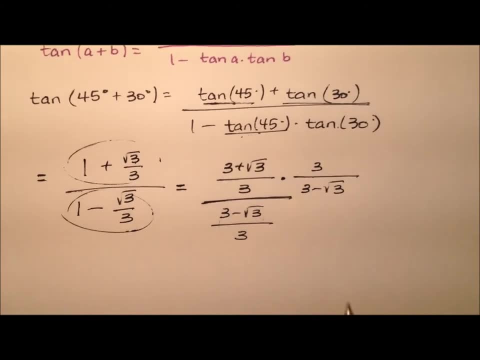 Okay, so when we're dividing fractions, really we're multiplying by the reciprocals. Let's flip that guy over, So we'll have three minus the square root of three there. and what's nice is those threes there cancel. So I'm left with three plus radical three for our numerator. 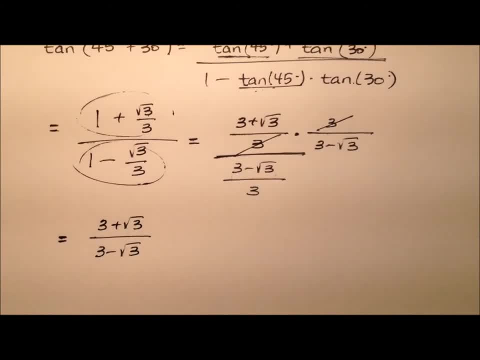 and three minus radical, three for our denominator. But of course we don't like having this radical or this square root expression in the denominator. So let's go through the process of rationalizing our denominator And in this case we'll do so by. 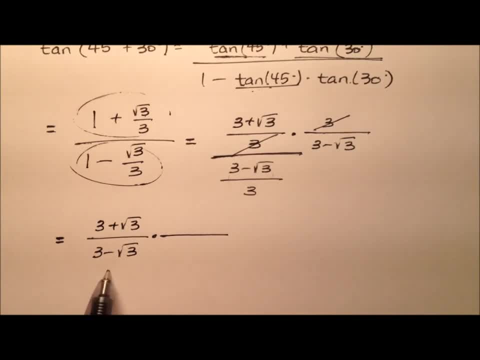 multiplying the top and bottom or the numerator and denominator by the conjugate of this denominator, And the conjugate just means let's change the sign in the middle, So we'll have three plus the square root of three. Okay, why this is so nice is because now. 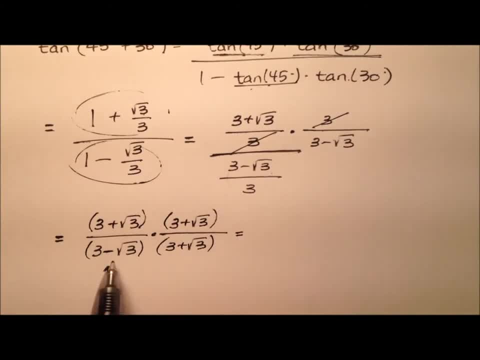 the denominator is set up as the difference of squares. factorization, where we have the same terms but one is minus and one is plus, So that will be a very nice multiplication. Okay, so for the numerator, it looks like when I go ahead and multiply these out, I will have nine. 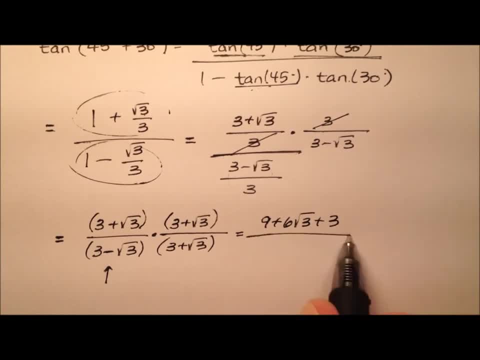 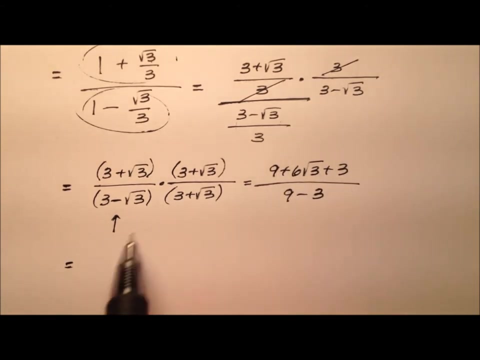 plus six, radical three plus three. when I go ahead and use that square of a perfect binomial formula And down here it'll be nine minus three. Okay, so let's go ahead and combine like terms. see what we have. So 9 and 3 will. 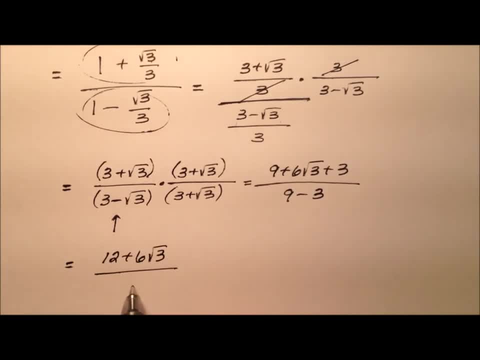 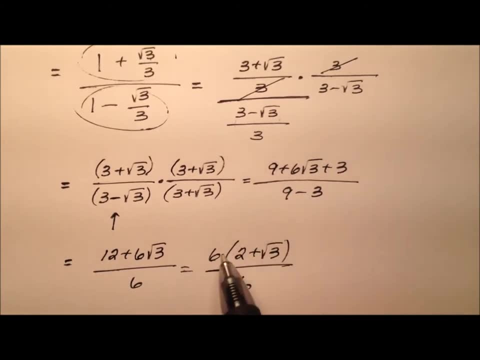 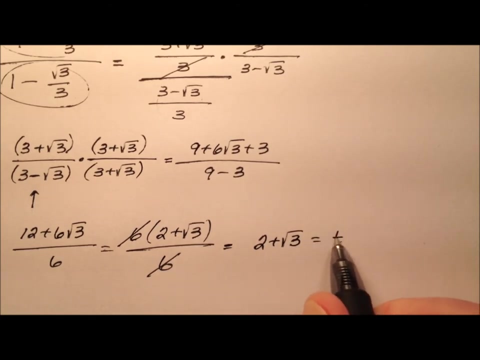 give us 12 plus 6 radical 3, and that'll be all over 6.. So in that numerator it looks like I can go ahead and factor out a 6 and those sixes will cancel, and so I'm left with 2 plus radical 3, and that will be the exact value for the tangent. 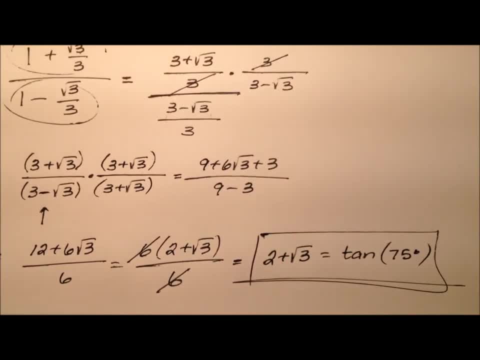 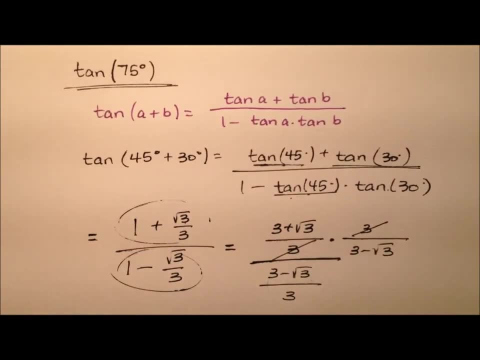 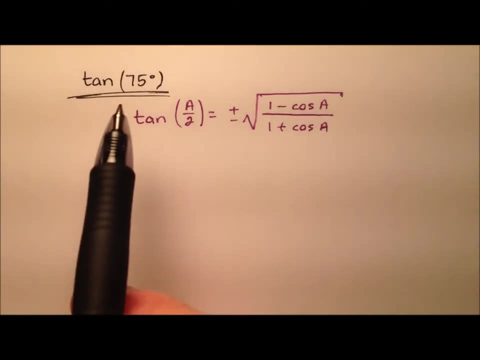 of 75 degrees, And in this first case we went ahead and got this exact value by using the sum identity for tangent. and here, once again, is that value. In this second approach, we will once again be looking for the exact value for the tangent of 75 degrees, but instead let's go ahead and use the half angle identity. 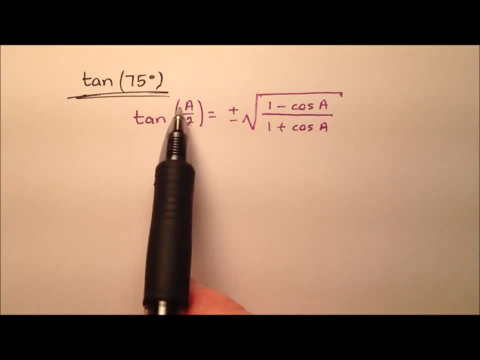 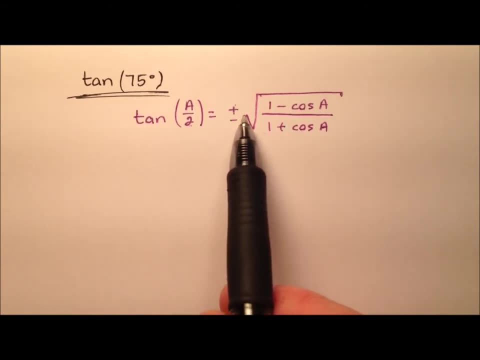 in this case. So we have here the tangent of some angle A and that's being divided by 2, and we have this formula that it's equal to plus or minus- and we'll talk about that here in a second- The square root of, and then we have this: 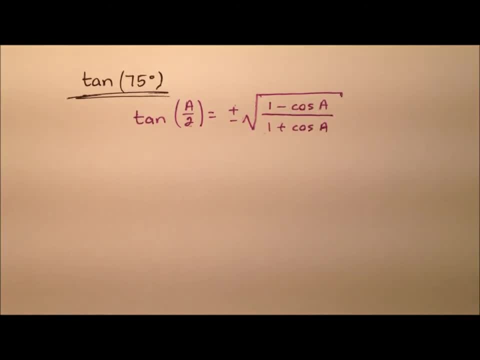 one minus cosine of A being divided by one plus cosine of A. Okay, so what should our value of A, in our case, be? Well, whenever I cut my value A in half, I get 75 degrees, so it seems like A needs to be a hundred fifty degrees, which you 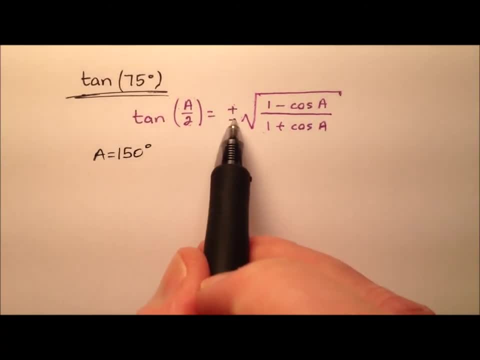 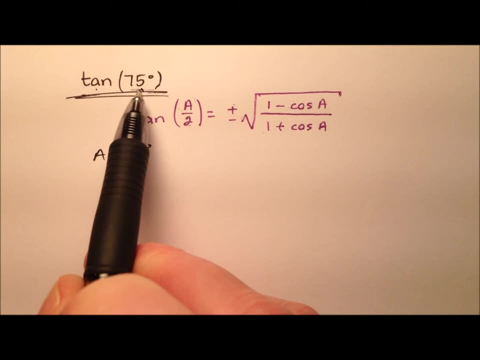 know it's twice 75 degrees. Okay, so how about this plus or minus? Well, 75 degrees resides in the first quadrant and tangent is positive in the first quadrant, So I will be considering this positive and ignoring the negative. Okay, so let's look at this now. I have the square root of 1 minus the cosine of 150. 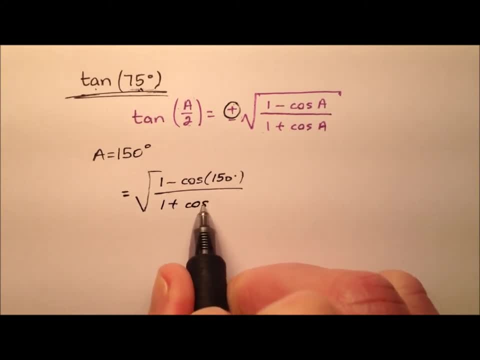 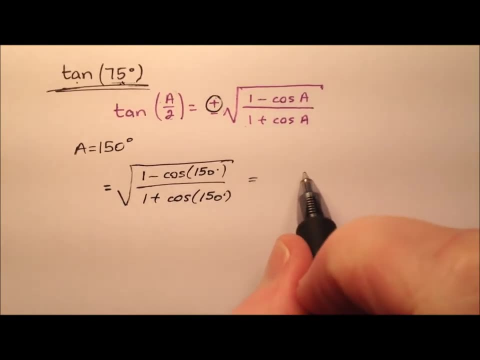 degrees over 1, plus the cosine of 150 degrees. Okay, so what is cosine of 150 degrees? Well, it's negative square root of 3 over 2.. So I'll have 1 minus negative square root of 3 over 2.. All of that will be over 1, plus negative radical 3 over 2. 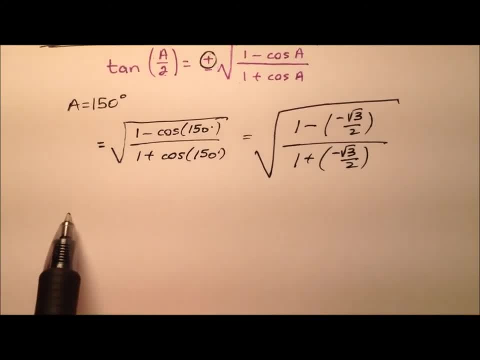 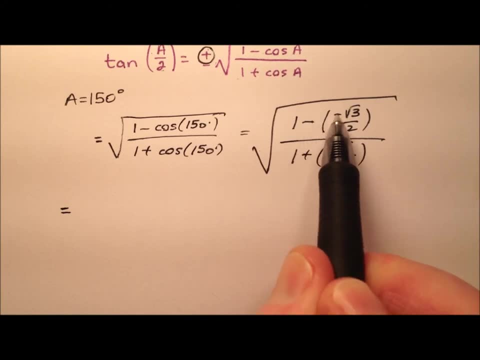 and, of course, all of that is under a radical Okay, so it looks like we have our work cut out for us to go ahead and simplify this. It looks fun, though, I think. Okay, so first of all, the minus and negative. that'll end up being a positive. 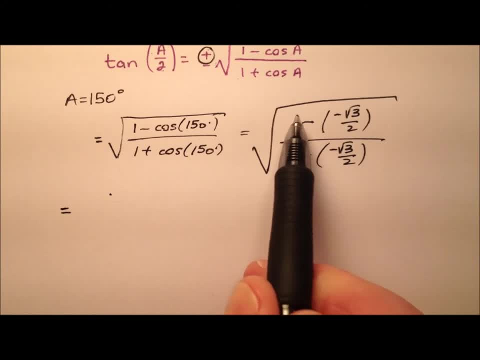 and then let's go and get common denominators while we're at it. This one will be 2 over 2.. So it looks like 2 plus radical, 3 over 2 for that numerator and the denominator. when we add a negative we can just say minus. and this one let's. 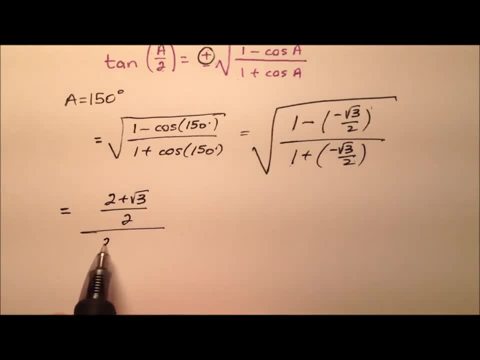 turn that into 2 over 2 as well to get our common denominators. So I'll have 2 minus the square root of 3 over 2 and all that is under that radical Okie dokie. So when we're dividing fractions, remember really we're multiplying by the. 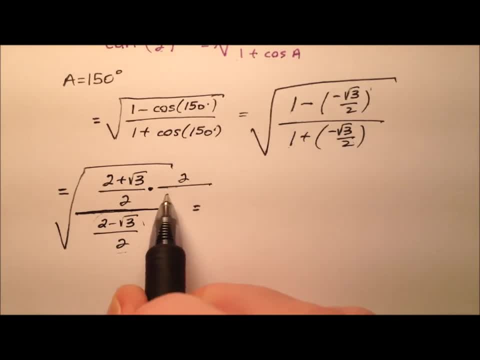 number of radicals. So I'm going to flip this guy over, get the reciprocal and do some multiplication here, and when we do that we see this is nice because those twos cancel out. So what I'll have is 2 plus radical 3 over 2 minus radical 3. 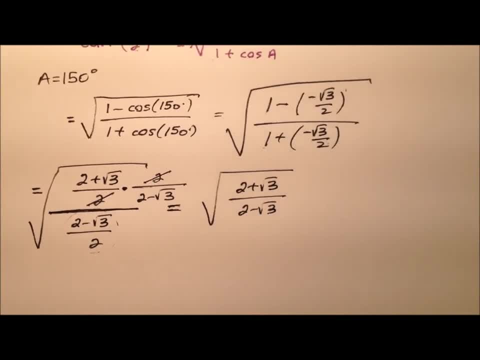 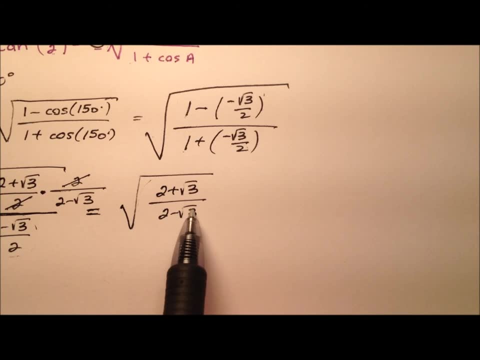 and all of that is under that radical. Okay, well, ignoring the radical for a moment and just looking at this radicand, we have this fraction and we don't have a square root expression in the denominator, So let's go through the process of rationalizing this. So when we do so, we'll just change the sign in the 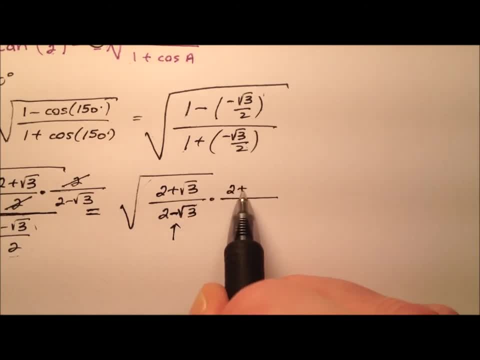 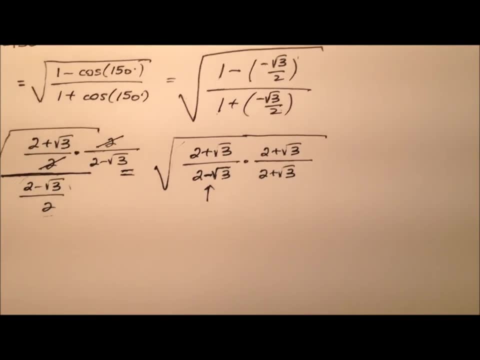 middle, and so we'll get 2 plus the square root of 3, and let's multiply that on top and bottom and of course all of that's under the radical. Okay, when I do that, some nice things are going to happen, because in the numerator 2 plus, 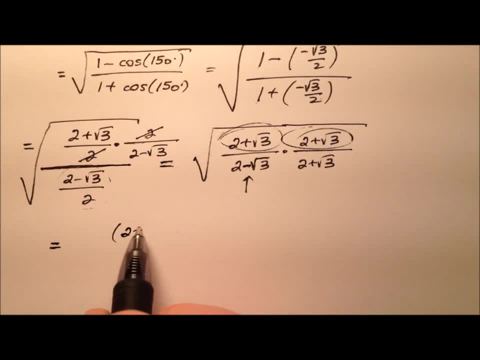 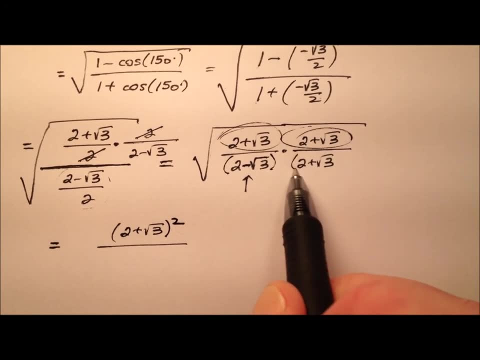 radical 3 times 2 plus radical 3 looks like we have a perfect square root right there and in the denominator nice things will happen, because when I multiply these, I'll get 4 minus 3, which is 1.. Okay, so the square root and the 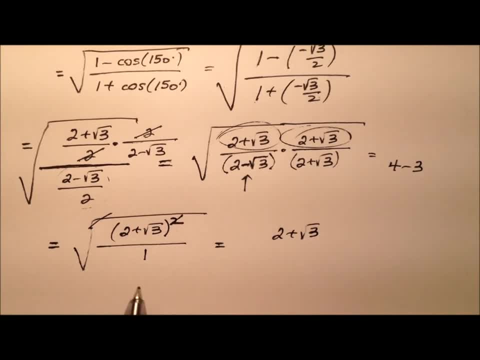 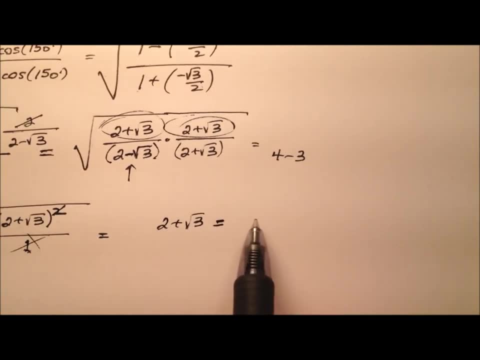 square will cancel out, leaving me with 2 plus radical 3, and of course the whole thing is over 1 and the square root of 1 is 1, so I can just ignore that critter. So 2 plus the square root of 3 will be the exact value for the tantalum. 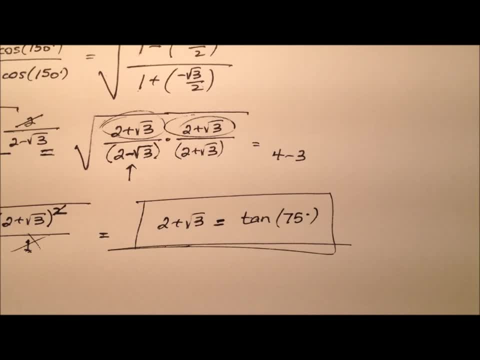 So that's the exact value for the tangent of 75 degrees. and if you recall from the first part of this problem what value that I get for the exact value for tangent of 75 degrees, Well, yes, again, 2 plus the square root of 3.. So we just saw. 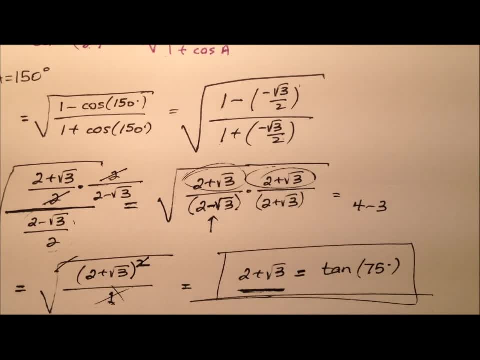 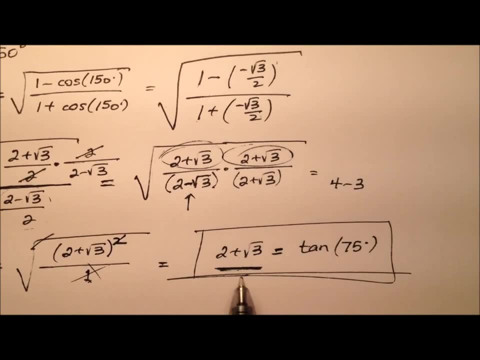 two ways that we can get this exact value for the tangent of 75 degrees: One using the sum identity for tangent, and in this one we did the half angle identity for tangent, Both of them yielding the same value: 2 plus the square root of 3..